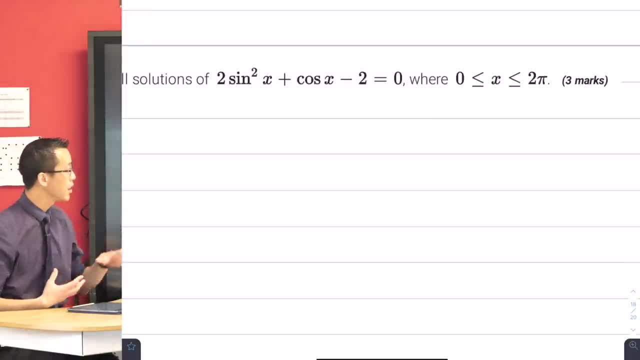 what looks like a fairly complicated mess. okay, Now, what we're going to do is turn this complicated mess into something much more, much more tame that we can deal with. okay, So does anyone have any suggestions? what might be a first step we could take? 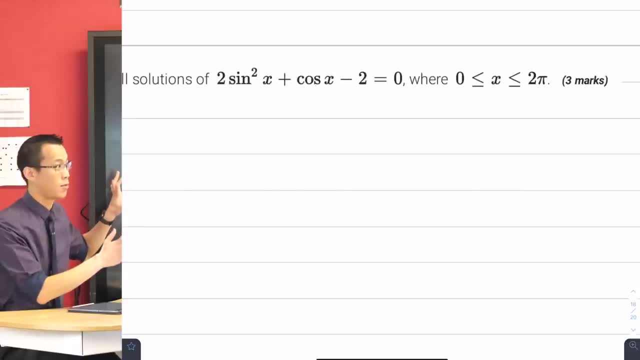 to make this better to deal with, because it's like a disaster right now, Sorry, Okay. so I want to get this into a form that we know That's for sure where we're going to head. I will point out for all of you- maybe some of you are already realizing this- 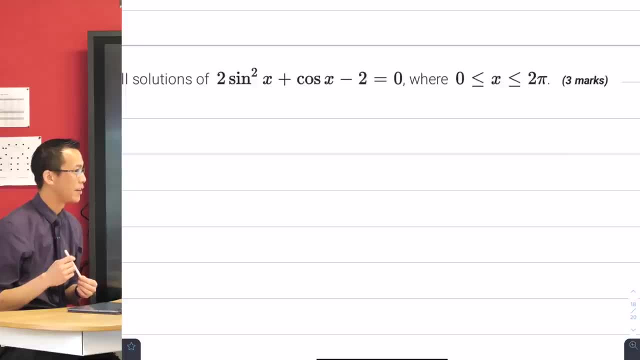 it's going to at least take me three or four lines to get to that point. okay, Do you want to suggest? what can we do practically? Okay, so you're looking at this constant here. Now I know this is going to sound strange, but even though it might initially look simpler, 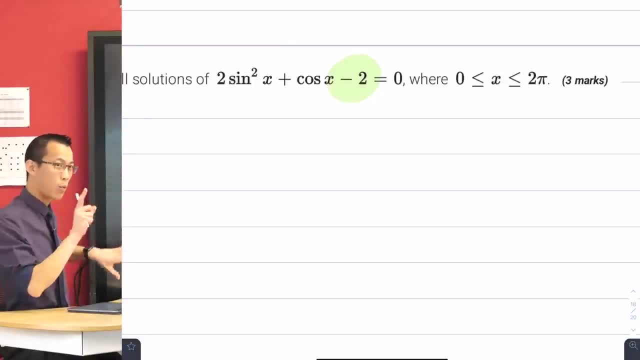 to add two to both sides and then we just have the trig stuff on the left-hand side. I will suggest that in this case, and in most cases like this actually, that will be counterproductive. It's good to keep everything on the left-hand side, okay. 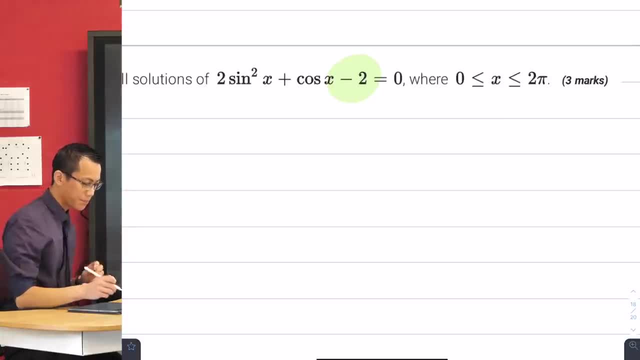 What are you thinking, John? Oh, whether sine squared X is to change that into like the identity, So it'd be like one line of code there. Okay, fantastic. So sorry, I think you were starting to head there, right. 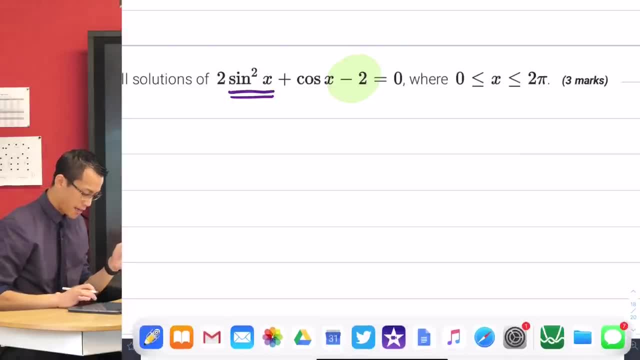 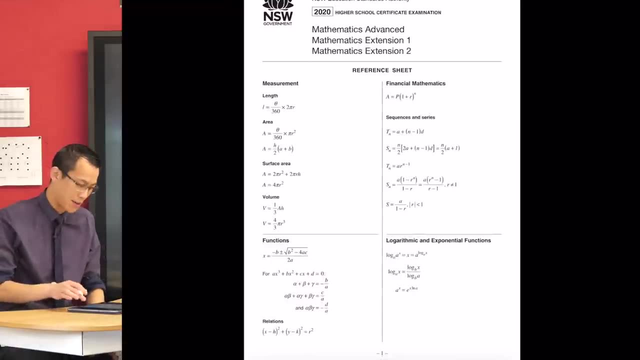 Now for those of you who are like: wait, what was he just talking about? If you have it there, go pull open your reference sheet. okay, Now here's page one. It's pretty simple stuff. We don't look at page one very much, to be honest. 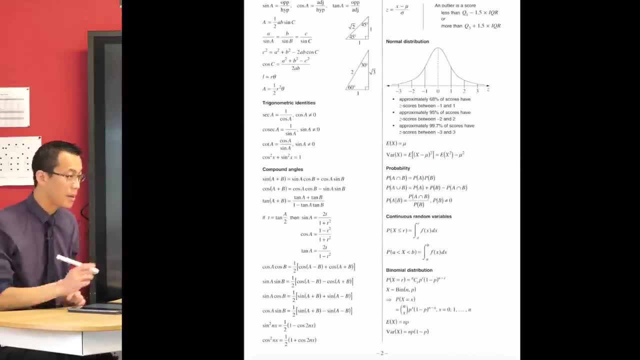 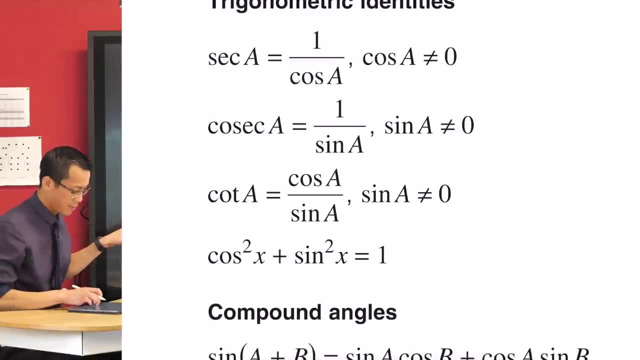 Page two. you can see a lot of the trig stuff comes in And what John's referring to is this guy here underneath trigonometric identities. So you can see right down the bottom: cos squared plus sine squared X Equals one right. 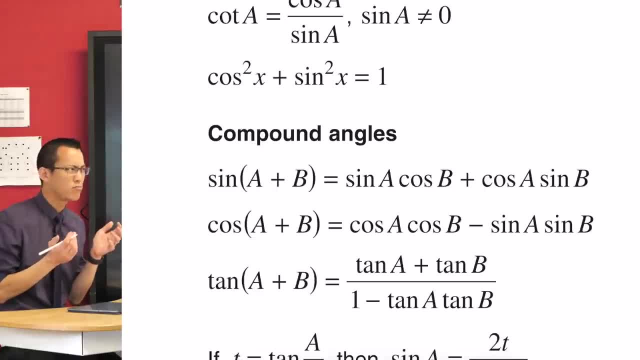 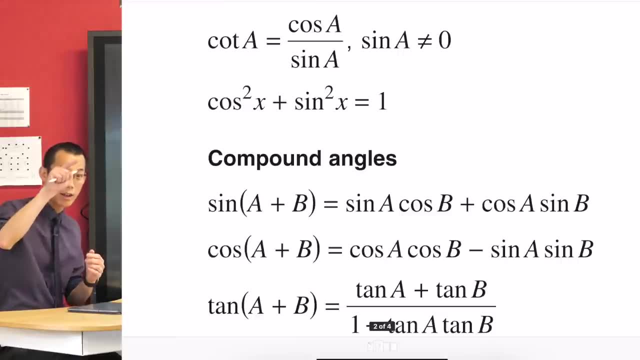 Cos squared X plus sine squared X equals one. This has a name, by the way. Does anyone know what it's called? It's not important if you don't know its name, but it's called the Pythagorean identity, Because if you've got a right-angled triangle, its sides can be sine cosine and one in the unit circle right. 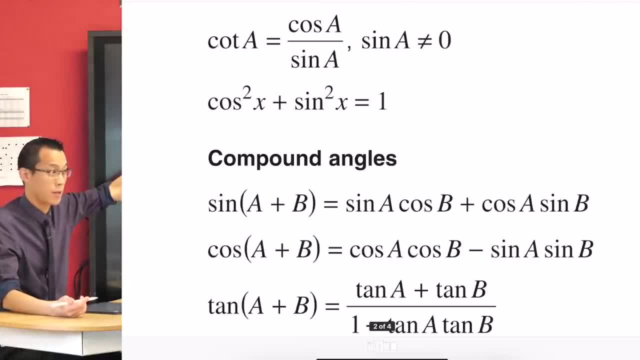 So this is literally Pythagoras: A squared plus B squared equals C squared, but with trig, okay. So how can we use this? Well, if I note, I'm going to say, I'm going to literally write this: 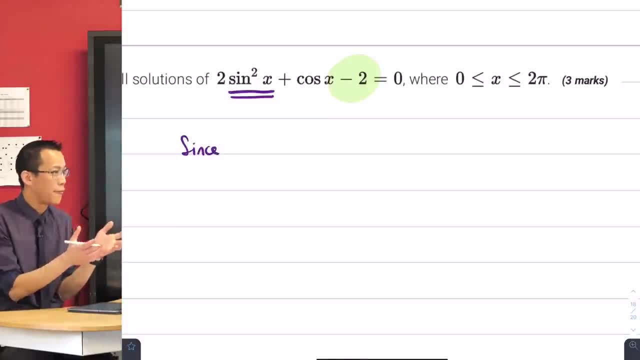 This first line, welcome, is probably not essential, but for the sake of our working, so you know what's going on, I'm going to write it for us, Since we have this identity up our sleeve: cos squared plus sine squared equals one. 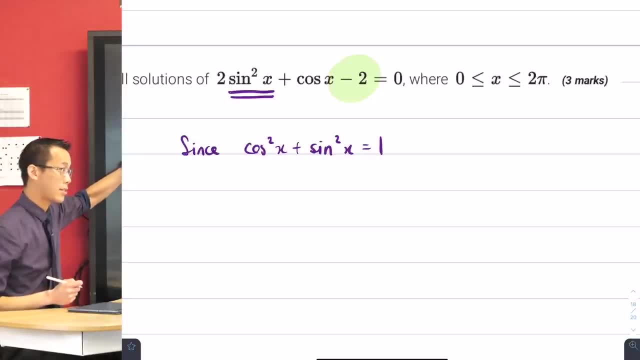 Therefore, as John suggested that sine squared X in the top line, I can substitute it if I just rearrange this line a little bit. right, I can say, since that is true, sine squared by itself is equal to- and John went straight to this line- actually one minus cos squared X. 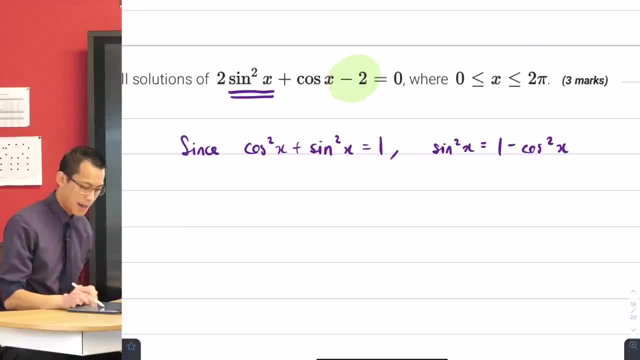 You okay with that, Right. So why is this helpful to us? Why is that a good substitution to make into our first line Any takers, Shane Barby, Fantastic. So part of the problem here is you've got sines and cosines mixed together, but we're going to make this all in terms of cosine and then we can work with it. 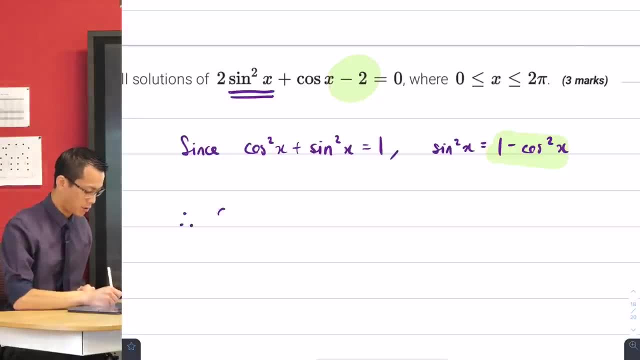 Okay, So let's go ahead. We'll make the substitution Therefore two outside of. I'm not going to write sine squared X, I'm going to write the substitution one minus cos squared X, And then I'll write the rest of the line. 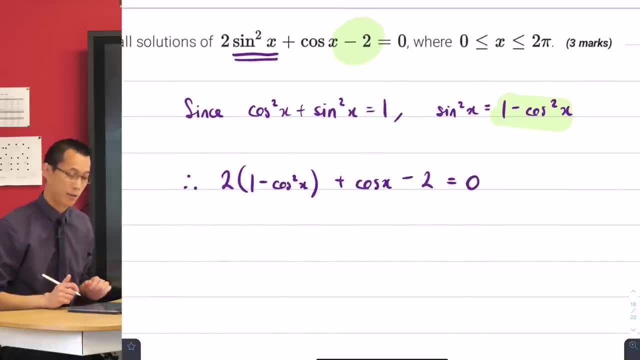 Okay, now this already looks healthier. right, I can start to expand some stuff. some stuff's going to cancel What happens when I expand. What do I get out the front? Two minus two cos squared X and then everything else right. 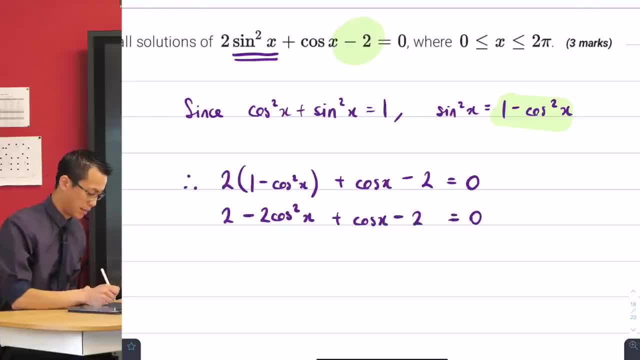 Now you can see, in this case it's just like super lazy, right, That two and that minus two. they're just going to cancel. So that's great. That's one reason why, you know, Soreng suggested we add two to both sides. 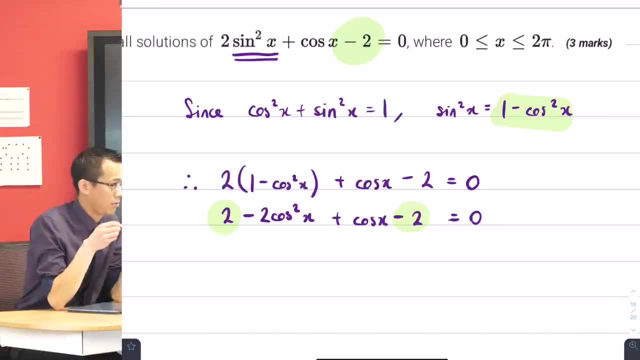 There was not really much point to doing that. Even if they don't cancel, though, right? Suppose you don't have to write this, but suppose it was like a three out the front there, right? Even if they don't cancel, you still want everything on the left-hand side, because why? 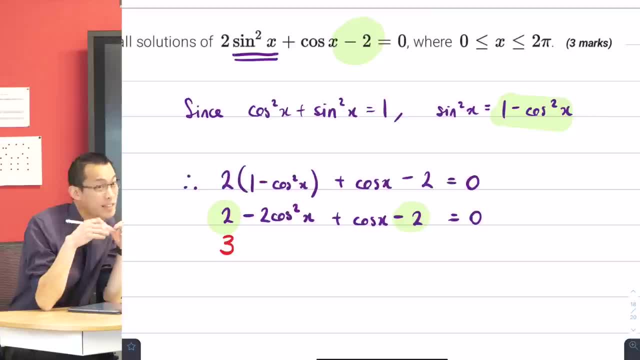 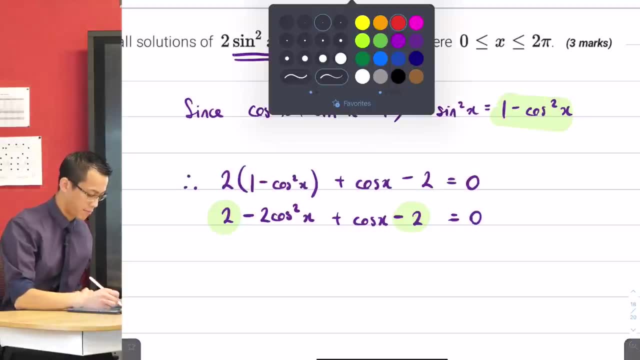 Why do we want everything on one side, Tyler? what do you think It's easier to work with? I'm going to factorize. eventually, You want everything on one side, so you can factorize. okay, In this case, the factorization is really quite straightforward. 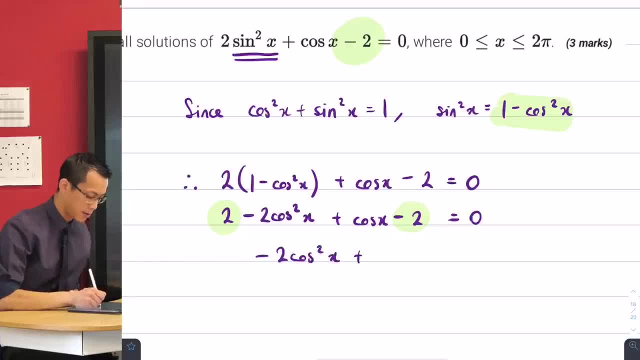 You've got minus two cos squared X there, plus cos X. What can I factor out? Cos X That leaves me with? this guy here is going to turn into one, and then this guy here is going to turn into minus two cos X. 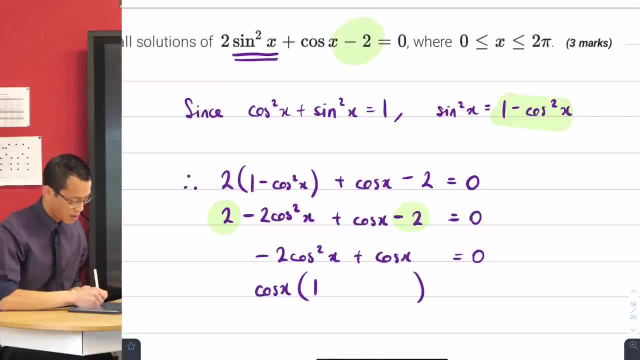 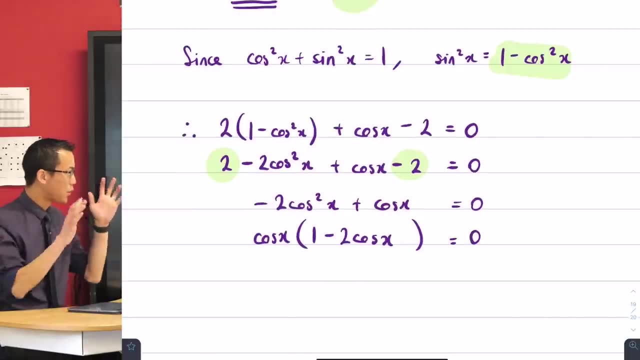 So I'm actually going to write that We usually write things with the positive first. So one minus two cos X, There we go. That's equal to zero. Okay, Now I feel like this is sort of mission, accomplishing that. now I can work with this. 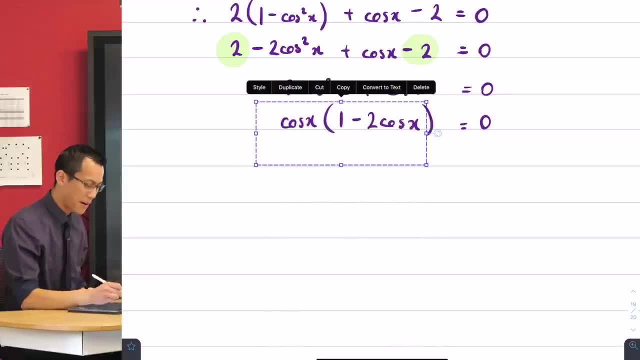 There are two parts to it. Sorry, that's bothering me. Let me fix that. There are two parts to it which we're going to solve independently, Two factors which we will get solutions from in each case right. So if you've got something times something and they equal zero, either of them could. 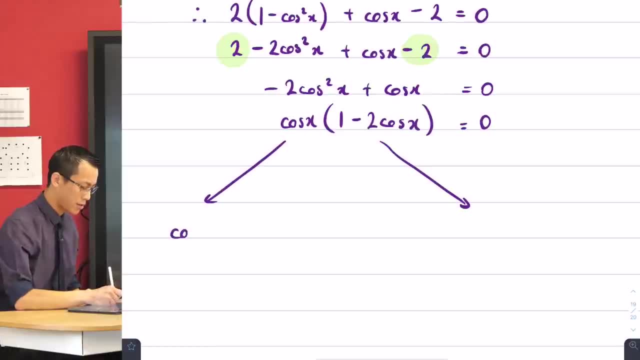 be equal to zero and you get solutions right. Does that make sense? So we can do this. If that's zero, then the lie will be true, And then also, if this is zero, the equation will be true. Okay, 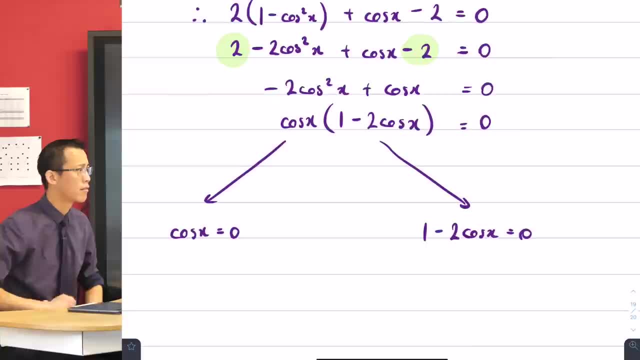 Now, just before I go any further, hands up. if you reckon I could take it from here, I could manage Hands up straight. Okay, can I give you a minute or two? You're going to get a bunch of solutions out of this, but I'm going to pause because I 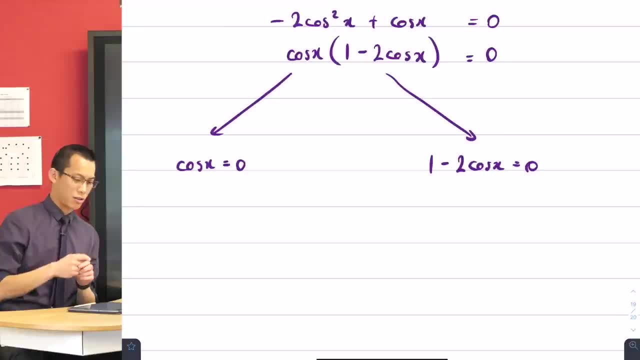 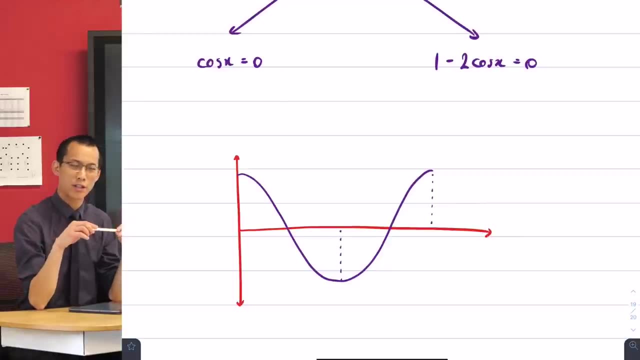 think we're at a much more comfortable point. I'll come around have a look and then I'll show you how we combine everything together. Okay, Off you go. Okay Now I was wondering around having a quick look, So let me bring you back together. 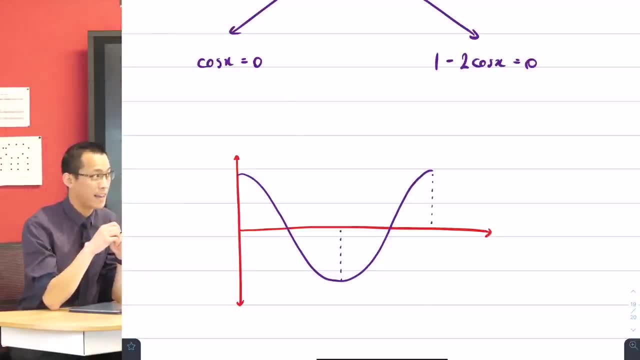 Now, the first thing I'm going to say is you should find four solutions. If you didn't find four solutions, Something has gone wrong. That's the first thing I'm going to say. The second thing is: I noticed a lot of you, like kind of a worrying number of you actually. 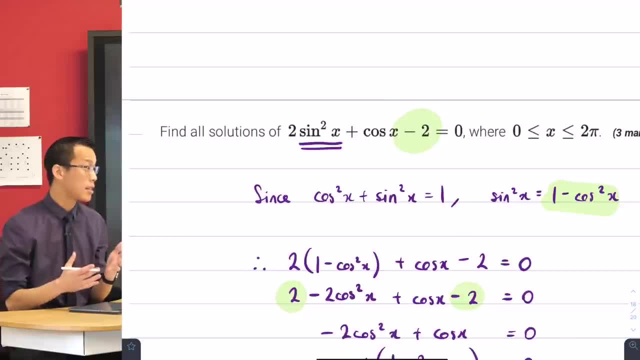 start to solve this problem, this one right here, and you started to think in degrees. Now I don't. that's not a bad thing objectively to do, because we're more comfortable with degrees. We can come up with those answers, especially for exact values, much more quickly and reliably. 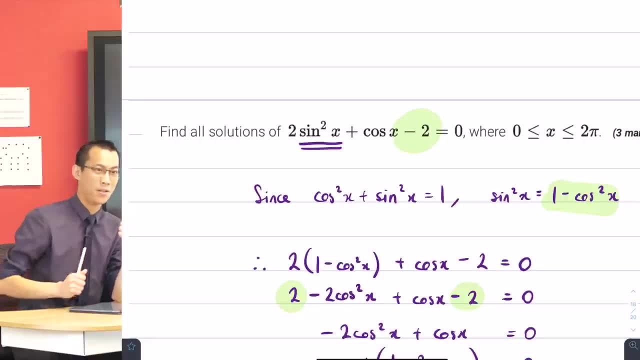 That's nice, But I'm going to give you all the warning Number one. I don't believe how many students think in degrees and then they forget to come back to radians. The domain is in radians. We must supply our answer in radians. 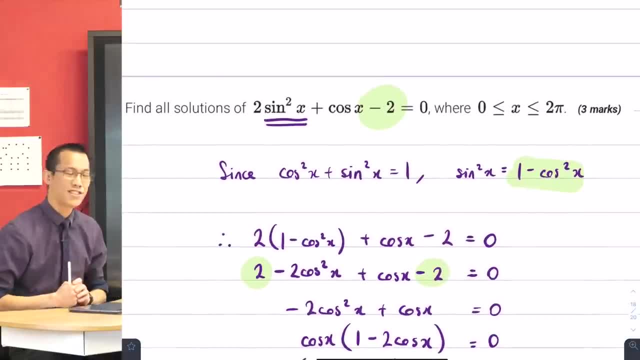 That's the first danger. The second one is you're just not going to escape radians Like you might as well start to get used to this thing right. It's kind of like living in a foreign country. to begin with, you're like I don't know how.